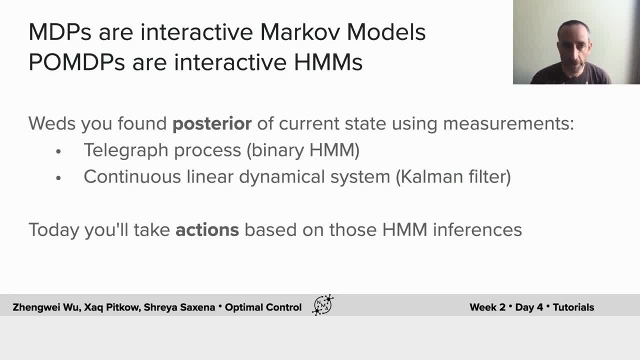 interactive Markov Models and you covered Markov Models in Tuesday. POMDPs are interactive Hidden Markov Models. On Wednesday, you found the posterior of current states using the measurements and we used two running examples: the Telegraph Process, which is a binary HMM, and the Continuous Process, which we use the Kalman Filter for. 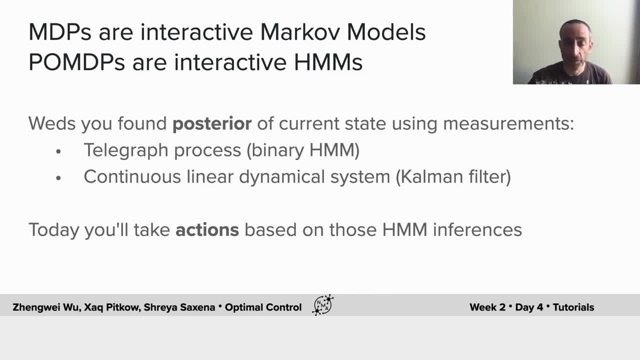 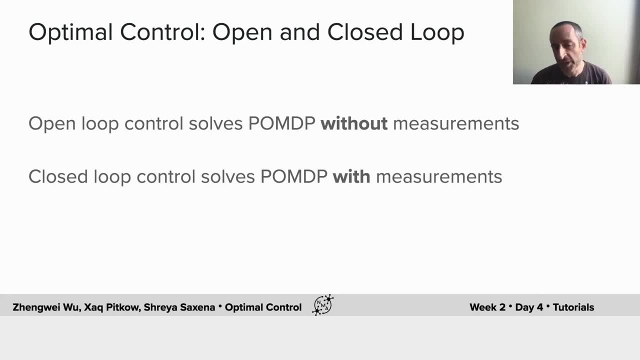 Now, today, you will take actions based on those HMM inferences. There's a distinction between Open and Closed Loop Control in Optimal Control, which is dependent on whether you get to make measurements of the current state. Open Loop, you solve the MDP under the assumption that you don't ever know what the future will hold. 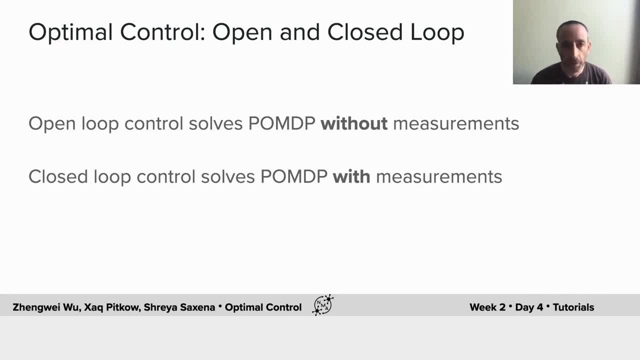 You just have to make a guess based on your starting point. On the other hand, if you keep measuring what the world is doing as you take actions, this allows you to have Closed Loop Control. So we will consider both of these in the tutorials. First we'll do Phishing. 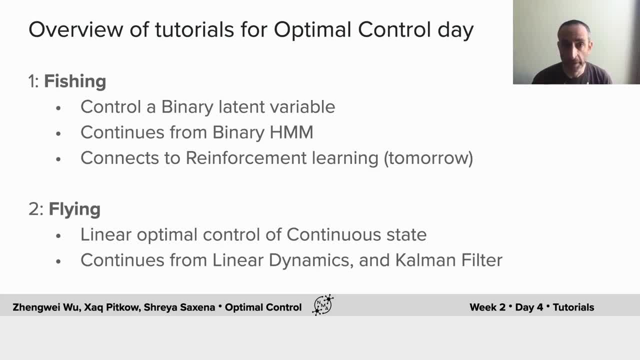 This is going to be our example for a binary Latent Variable or a binary POMDP, And this will continue from your binary HMM from yesterday and it will connect to reinforcement learning for tomorrow. The other example in Tutorial 2 will be Flying, where we will use 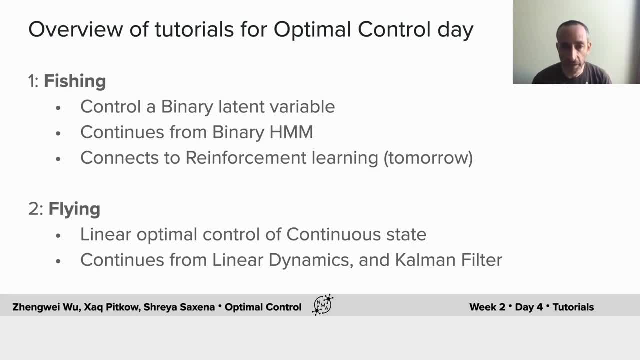 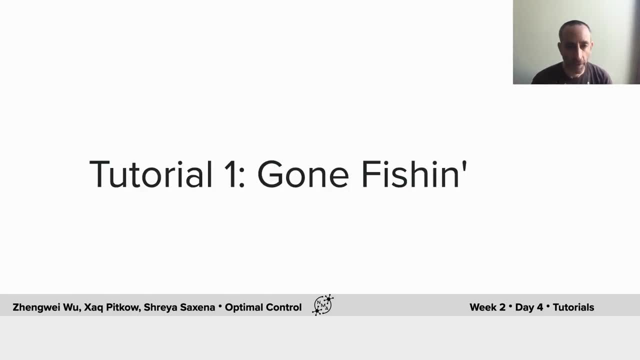 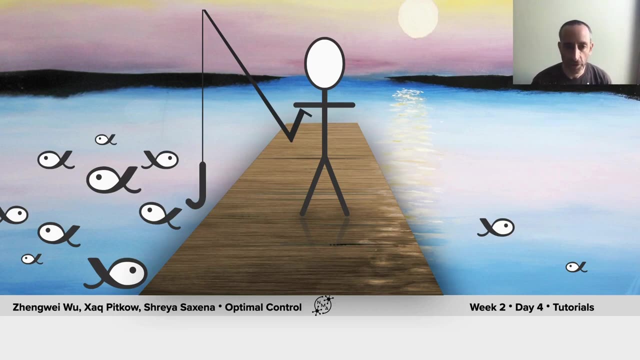 linear dynamics and a linear continuous state with Gaussian noise, and that will continue from the Kalman Filter that you learned about yesterday as well. So now we'll begin with Tutorial 1, Gone Phishing. The setup here is that you're trying to catch fish and there's a school of fish which swims. 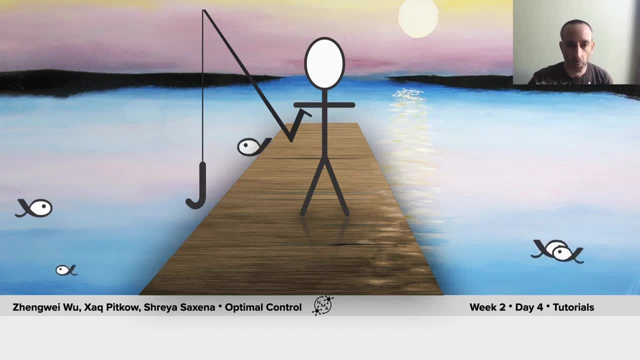 back and forth between the two sides of a dock, And when you're on the right side of the dock you catch a lot of fish. but then, when the fish move- now it's rarer for you to catch the fish On the other side- you can move over and now you catch more fish until they decide to leave again. 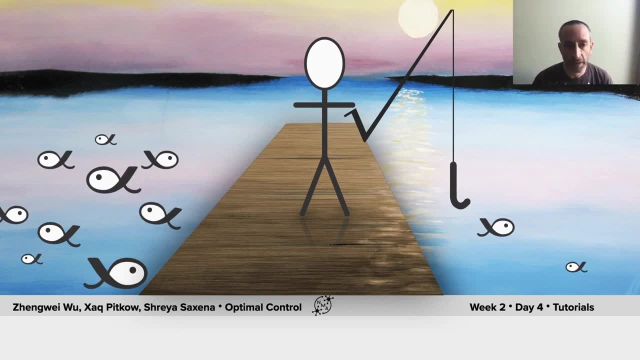 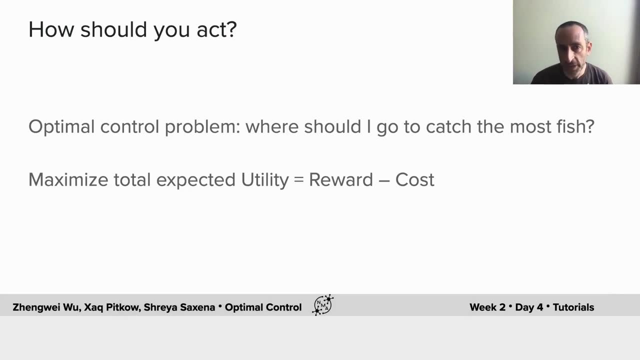 And so your control task is to find out where you should be at any given time, When should you stay on one side, fish longer, and when should you switch. How should you do this? Well, this is an optimal control problem. Where should I go to catch the? 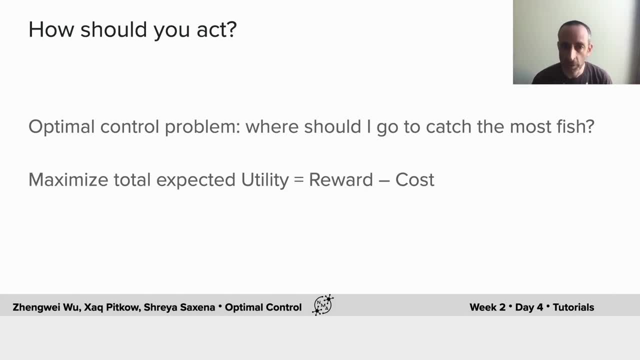 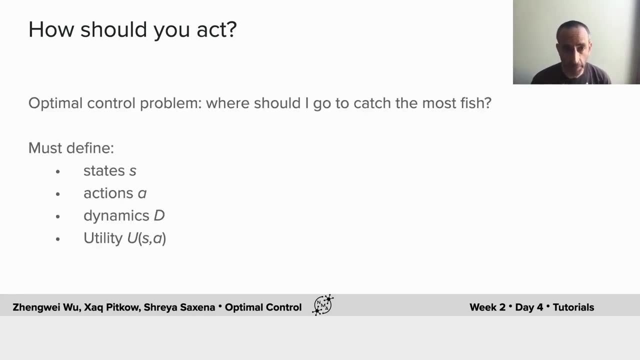 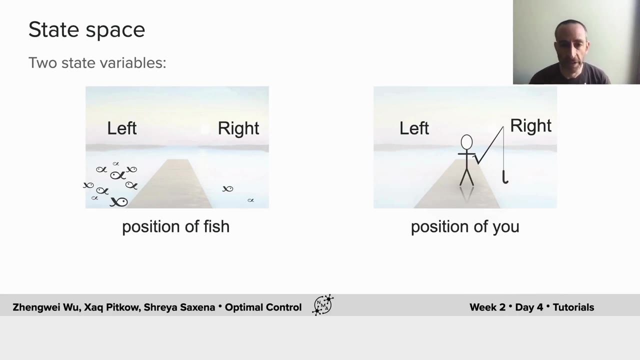 most fish, And the goal here is to maximize the total expected utility, which is really the reward minus the cost. And in order to define that problem, we have to define the states, actions, dynamics and utility. The state space that we'll choose in this problem is two state variables.